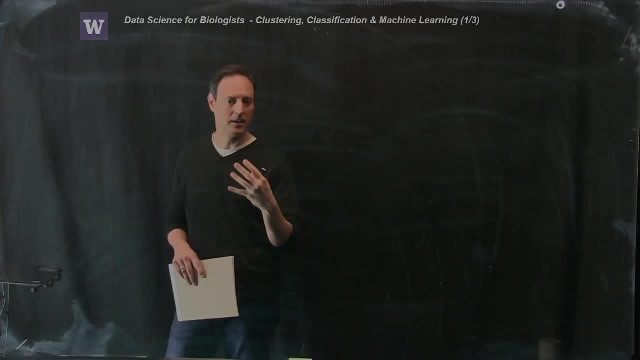 tasks where you identify a new piece of data and you classify it as something that you know. you may also want to do some kind of looking for clusters in your data. Maybe you don't know much about the data and you want to just try to understand. are there patterns? 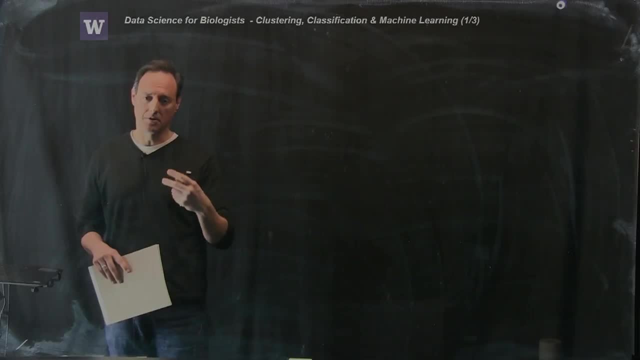 of the data which you don't know about and you're trying to discover. And there's also ideas of regression which are: can I actually take my data, think about doing curve fitting to that data so that I can make predictions based upon that data and apply it to new data? 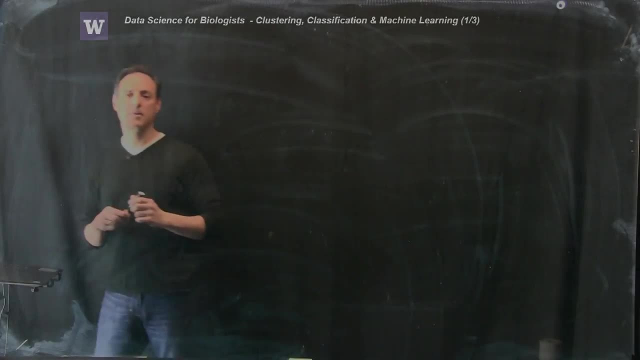 Okay, so we're going to talk about some of the key ideas, And some of the key ideas revolve around this idea of learning from your data, So we might think about this as generically learning, or you might want to just call it data mining, And the idea is to think about 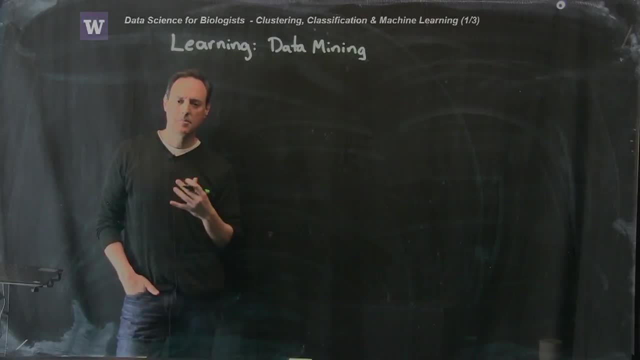 taking that data, looking for structure in the data, and it comes in two broad techniques, And I'm going to go through both of them here now, which are: and, in fact, in the series of lectures, what we're going to do is cover a lot of the key technologies, a lot of the 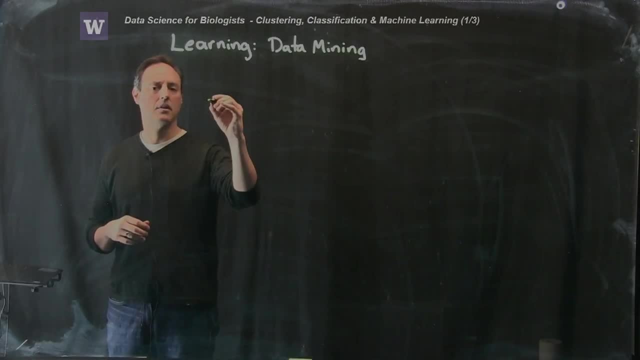 key methodologies around these methods. So the first thing I'd like to highlight is a this idea of unsupervised learning. So the idea here is just as it sounds- is that you're going to basically generate an algorithm on your computer that's going to look for patterns. 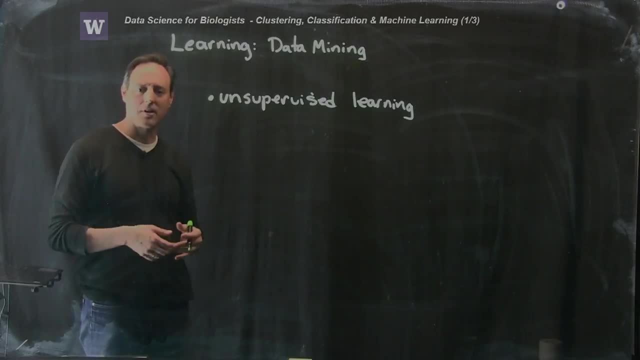 in the data. You're not going to label any of the data, you're not going to tell the computer what kind of data it is. The goal of the algorithm itself is to discover these patterns in the data without you being the architect of that discovery process. Another: 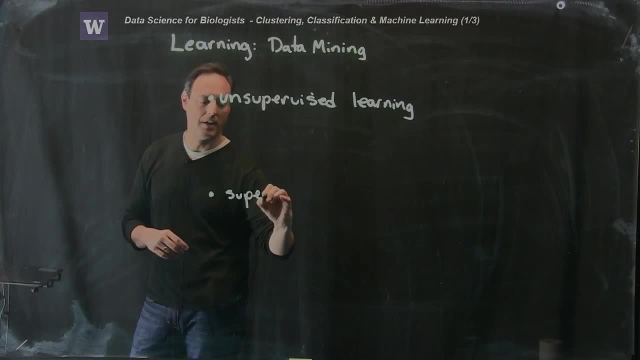 type of data analysis is called supervised. Supervised learning is a little different. This maybe assumes that you know something of your data, and then the idea would be is to capitalize on what you know, And perhaps you even can classify some of your data. You might think about pictures of dogs, pictures of cats, And if you have cats and 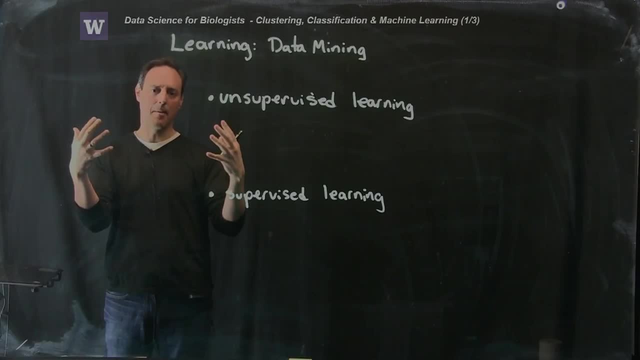 dog pictures. how would you take these dog and cat pictures? and let's say, maybe you have a hundred dog pictures and a hundred cat pictures. I'd like to do a training algorithm so that if I give you a new picture of a dog or cat, your computer could actually classify. 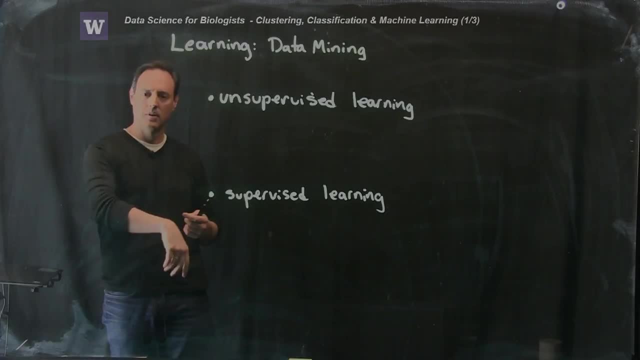 that as a dog or cat. And that's the idea of supervised learning- is that you're going to label data ahead of time in this process so that you can make future decisions based upon that. Now, interestingly enough, these two algorithms are trying to do different things In unsupervised. 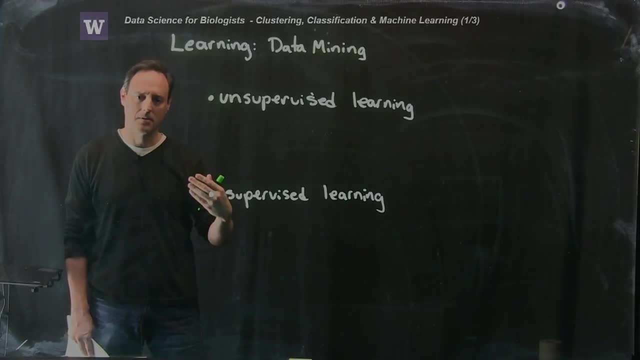 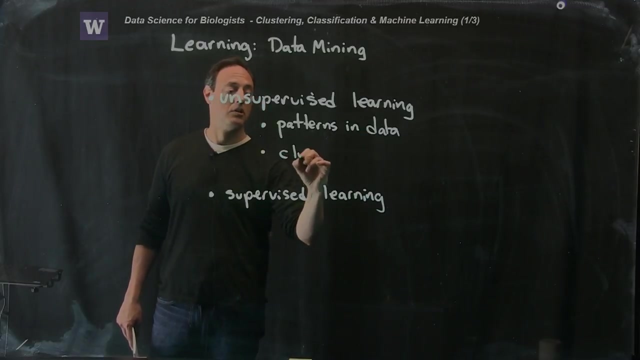 learning. the goal of this is to look for patterns. The goal of this is to take your data and discover clustering in the data in some kind of space. So unsupervised learning is really about patterns in your data. So you can either look for patterns in your data or looking for clusters in your data. 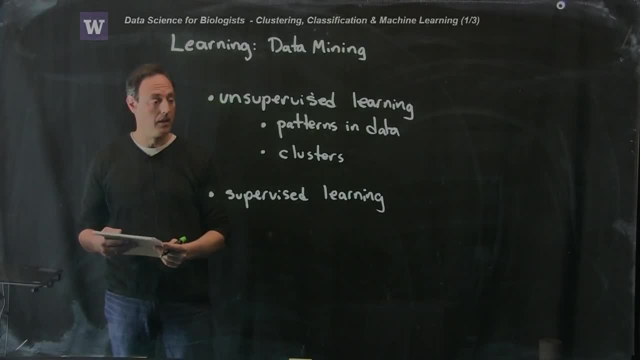 And we'll show some examples in a little bit with this. So this is this data mining operation. You don't know anything, you're just going to put it in there, go look for things and hope that, in fact, you can do a good job in finding those things. 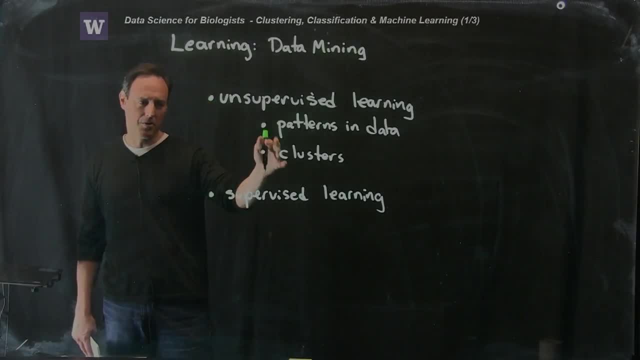 Supervised learning is different Because in some sense it's already assuming that that you might have clusters. The cat-dog example is one where you say: I have pictures of cats, pictures of dogs, and so I already have clusters, I already know that I have dogs. 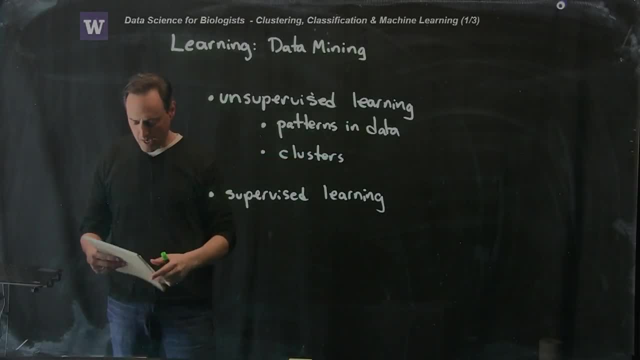 I already know that I have cats. So you are the expert in the loop And then, sort of in this idea, you are providing labels. So you're gonna label the data ahead of time and you're gonna give this data some okay, I have dogs, I have cats. 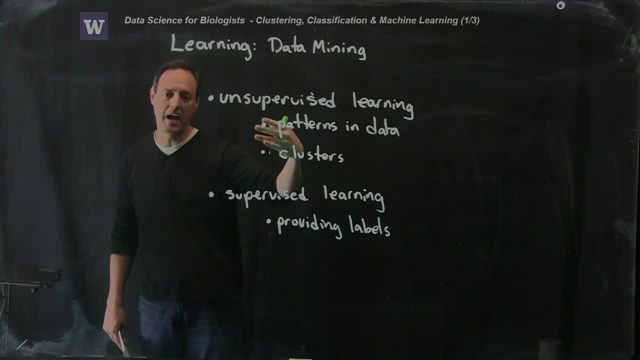 I labeled them all. I know what they are, and now the idea is to make use of that and if I give you a new dog or a new cat, can you actually label it correctly yourself, or how can I write an algorithm to do that? 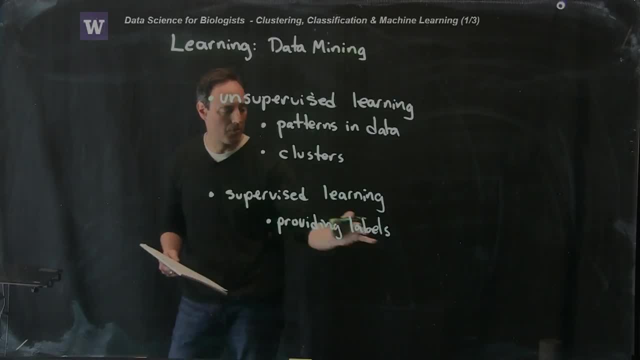 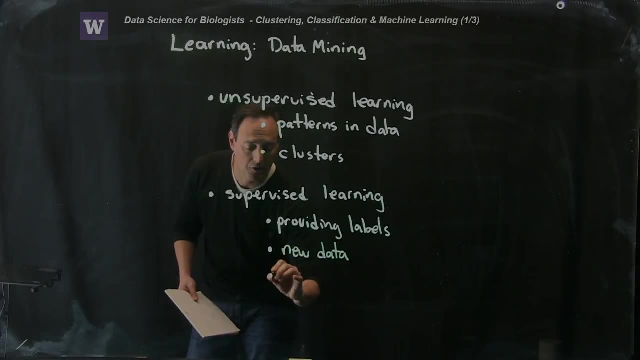 Okay, so this is gonna invoke the idea of providing labels for data, and then you're gonna try to see what you can do with new data- How do I label new data? And so there's gonna be this training phase and then a test phase. 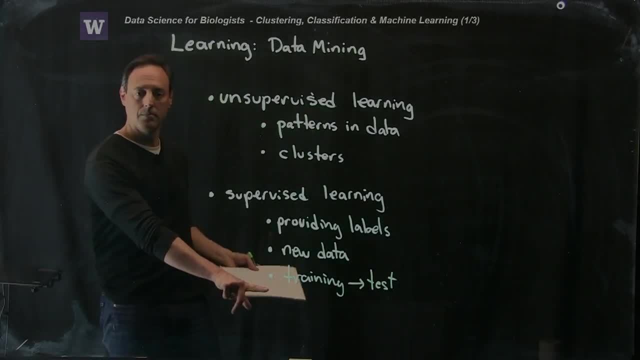 So the training algorithm, the idea behind the training, is to sort of take these ideas, use the fact that you know what cats and dogs are, so you can train an algorithm to recognize what the key structures of the data are based upon your expert in the loop opinion. 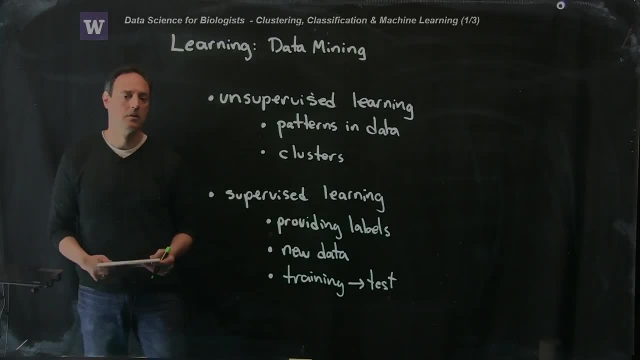 and then you can go test new data and see how well you did okay. So one idea, then, is: clustering is happening. here in supervised learning, You're looking for clusters, you're looking for patterns in the data. In contrast, here in the supervised learning, 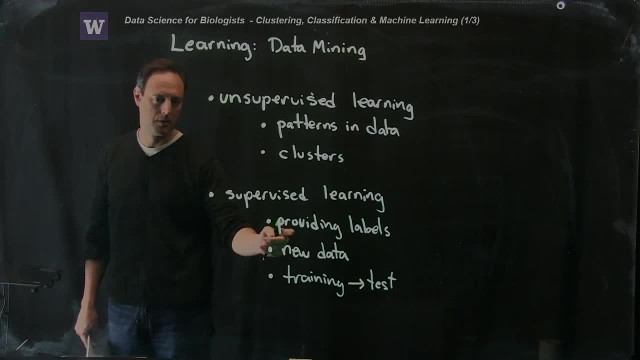 you're not necessarily looking for clusters. you've already told it by providing the labels what the clusters are. So what you're kind of trying to do in this case here is actually do classification and also regress. So the idea behind classification and regression is: if I can do classification, 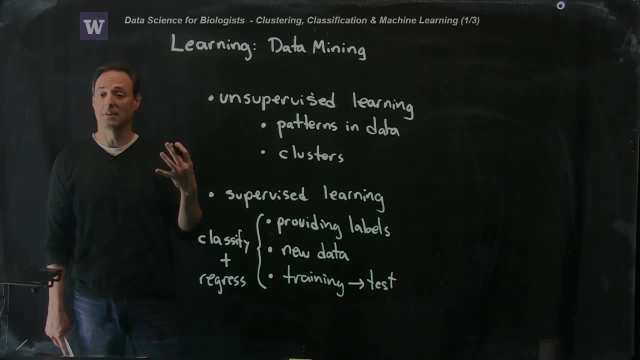 I can find some kind of regression curve or some kind of basically best least square fit type curve to the data. it doesn't have to be linear. that actually explains this classification data. So that's kind of the big picture thinking behind these two learning algorithms. 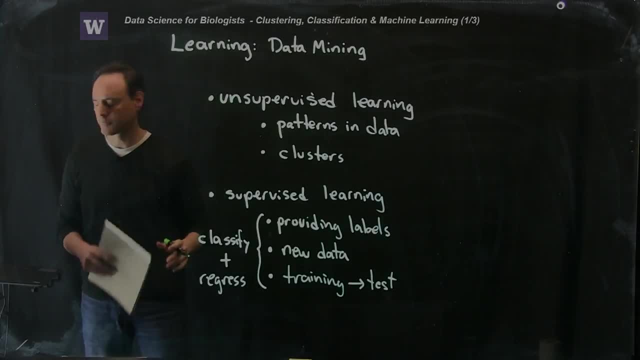 And we're gonna hit a lot of the common algorithms used for both. Now, before we get to that, though, what are the advantages and disadvantages? Well, in unsupervised learning, the disadvantage is that you don't give any information, or expert information or knowledge to your algorithm. 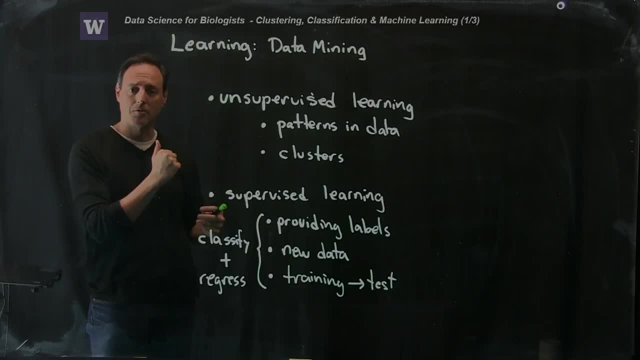 So it has to figure it out all by itself. It may not even know the right number of clusters. Suppose, for instance, you have dogs and cats In an unsupervised algorithm. the data's not gonna if you're just letting this thing look for patterns. 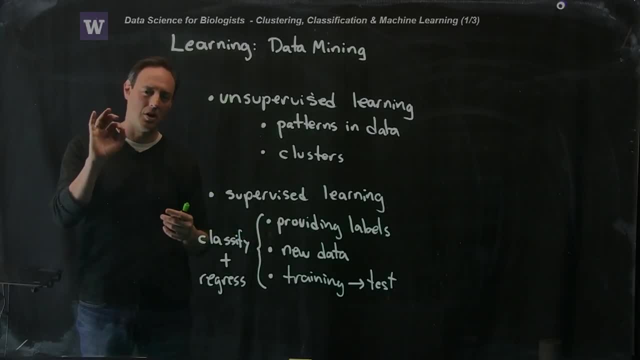 in the data. it may not know that I'm looking for two distinct clusters: dogs and cats. Okay, so that can be a drawback here, and it's actually typically the Achilles heel of this method, And this is why you want supervised learning. 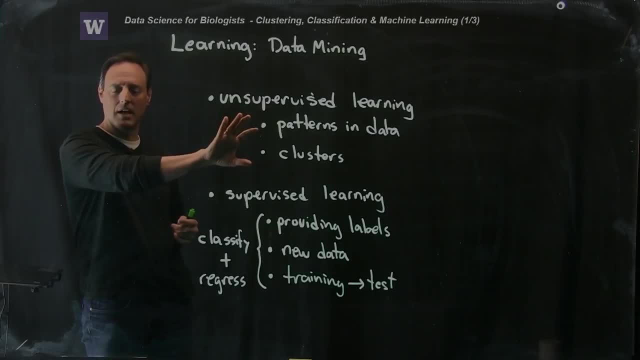 because here you're kind of telling it what to look for ahead of time, or you'd like to, but the unsupervised learning doesn't have that capability unless you enforce it yourself. okay. The supervised learning, on the other hand, 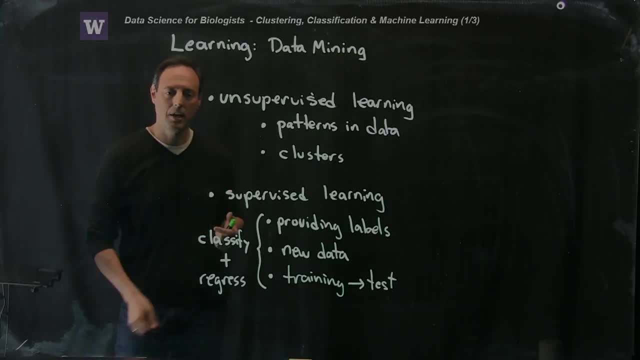 already assumes the kind of things that you're looking for, which is you're gonna give it a training set and you're gonna provide labels. So maybe you already have two data types- dogs, cats- and so it already knows it doesn't have to look for. 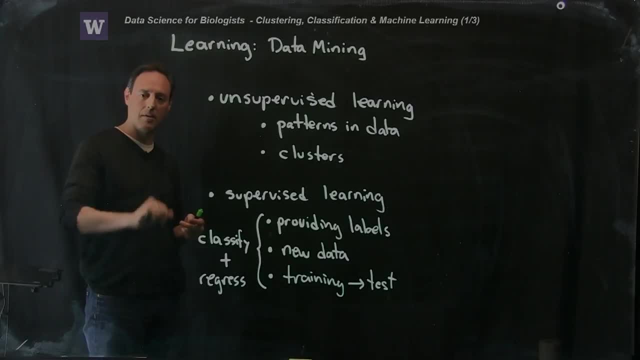 how many clusters am I looking for the data? It already has that information and you gave it to it. Okay, and not only that, you gave it expert opinion to start building a training set off of this thing here, And so there's some kind of advantages. 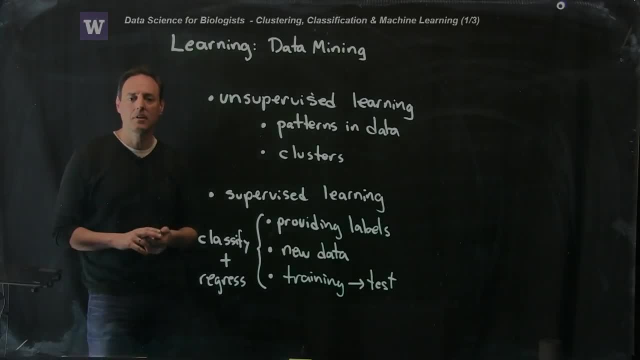 with supervised learning. but the disadvantage of supervised learning, of course, is that there's a long-time training stage. sometimes You take a lot of data and if you want good classifiers, oftentimes you have to go through a long-time training stage. 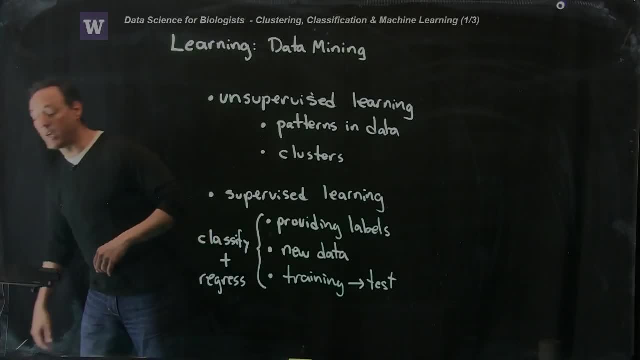 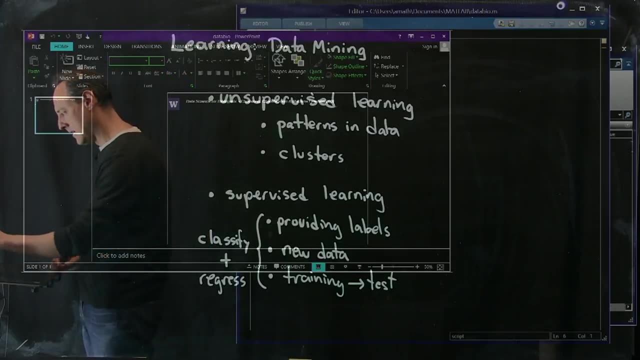 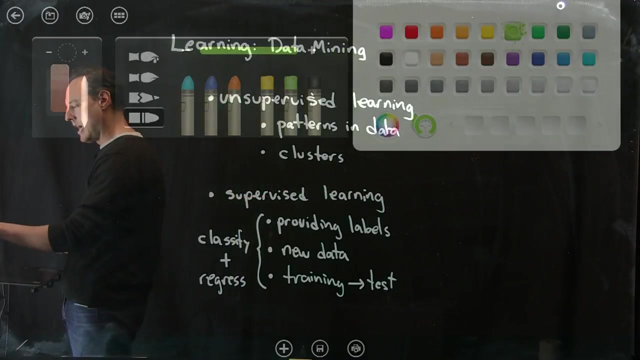 in other words, to do the classification. Okay, so let me show you an example of what this might look like. So, and then we're gonna program the MATLAB. Okay, I'm gonna do this here. I'm gonna show you what this might look like. 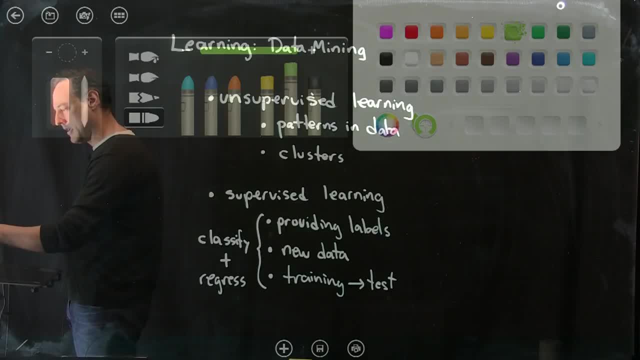 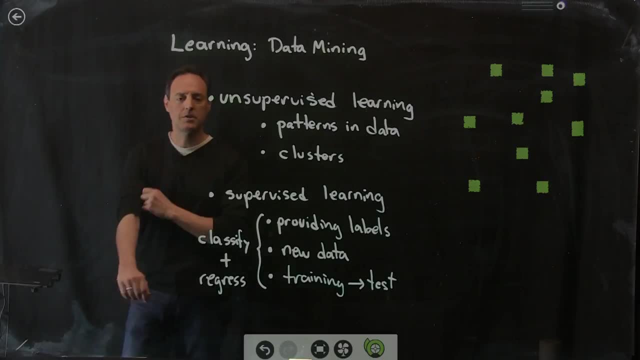 Let me come over here and pop some data out for you here. Okay, So this could be some kind of data set where I'm looking at in some abstract representation. here's a bunch of green squares, and they could be, let's say, dogs or cats. 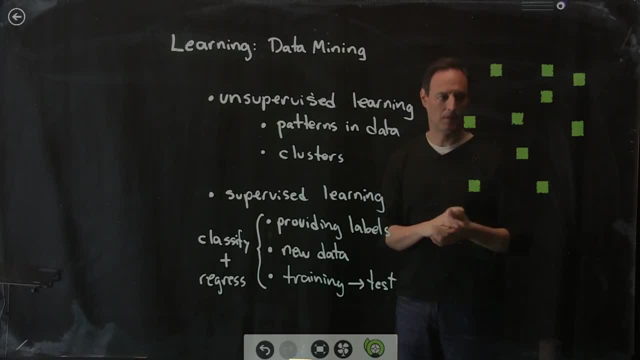 or some kind of projection of dogs and cats into a two-dimensional space, right? So it's kind of nice. They kind of are here and clustered, and each dot would represent a different dog, for instance. So that's kind of a sampling of data that you might have. 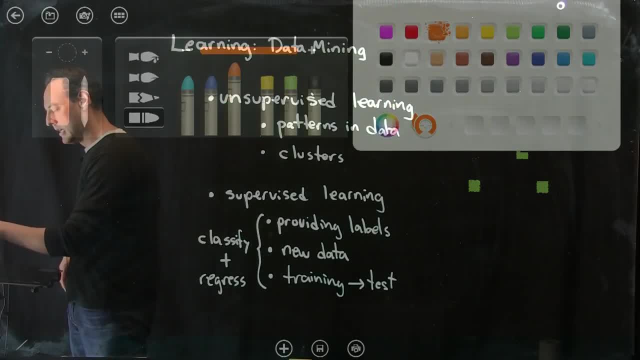 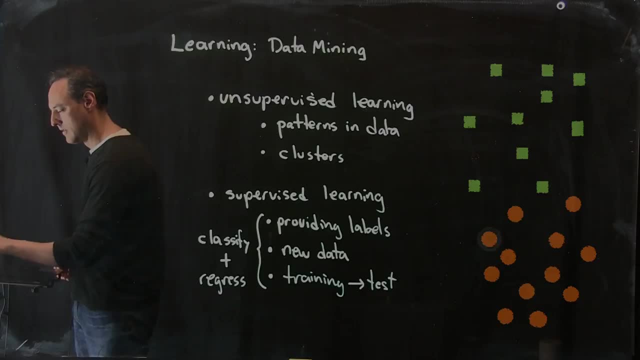 And then you could also have a different type of data, And let's represent this in orange. sure, That sounds great, And suppose those are your data sets. So now what you see is you have these two data types: You have the green, you have the orange. 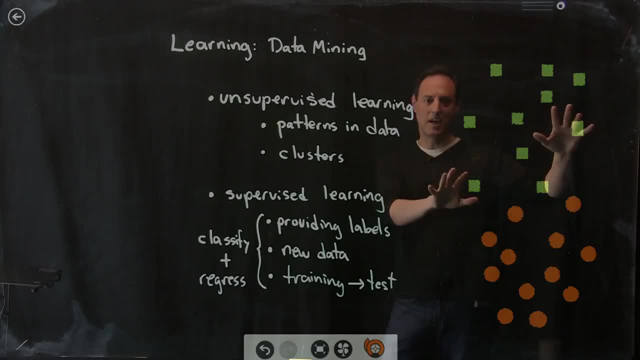 and of course here it's almost trivial to say that they're different. right Here you can say: well, there's the green and the orange. I see clearly the difference, And the idea then would be to say, oh, what I will do is form a cluster around the green. 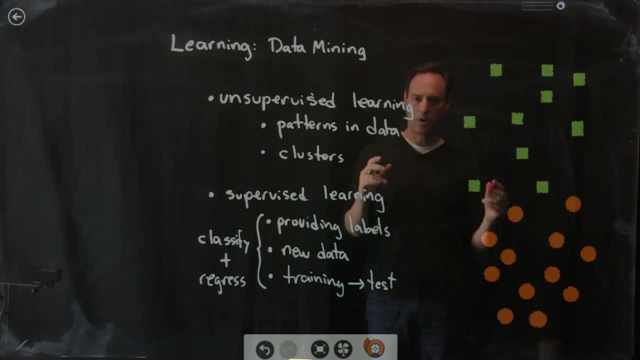 a cluster around the orange. okay, So that's one operation that you might start to think about doing. is that you can easily do this classification task? Now let's talk about how it relates over here to the unsupervised and the supervised learning. 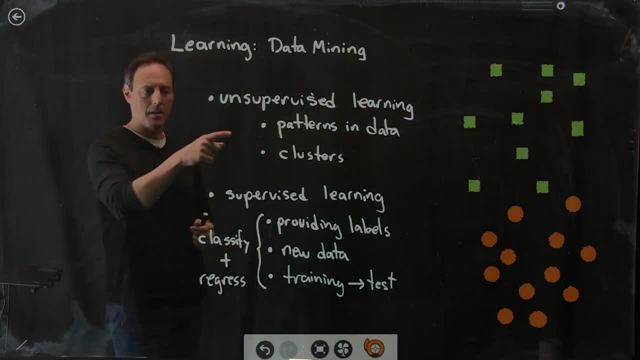 If you're in an unsupervised learning algorithm, then you don't even know that there's two things, two objects, let's say green and orange dots. So ahead of time, you're gonna have to make some decision. You're gonna say, hey, I'll train my algorithm. 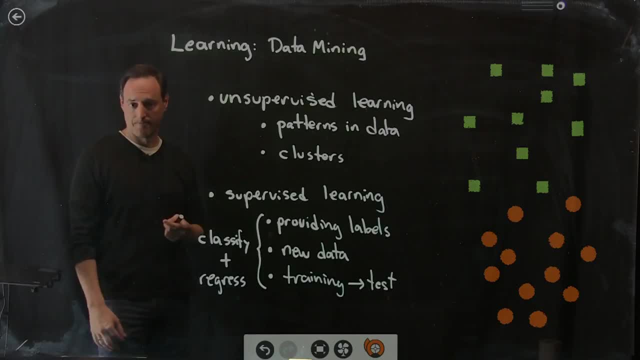 and say: go, look for two clusters, for instance, And in that case, if you pick two- and clearly there are two- what it would do is start to figure out: can I form two clusters? And the idea would be: here's a cluster one. 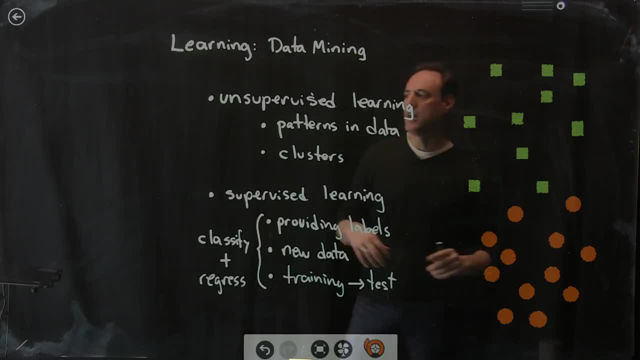 and here's a cluster two. okay, Now the unsupervised learning. that's all it essentially does, is it provides a way, a principled way, to do that clustering. Now, what's interesting is you can use the unsupervised learning. 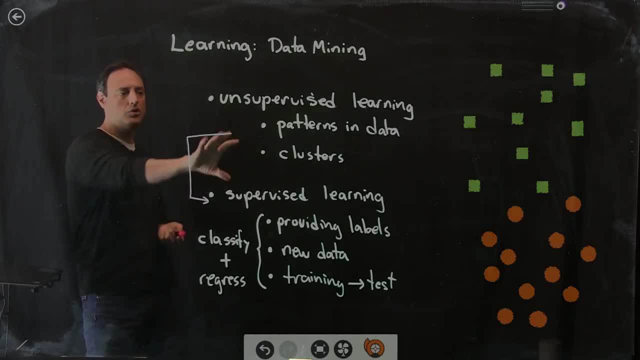 and then feed it into the supervised learning, Because once you have the clusters, it's equivalent to providing labels. Now the supervised learning. what it tries to do is to say: well, I have this data, I've given expert in the loop opinions. 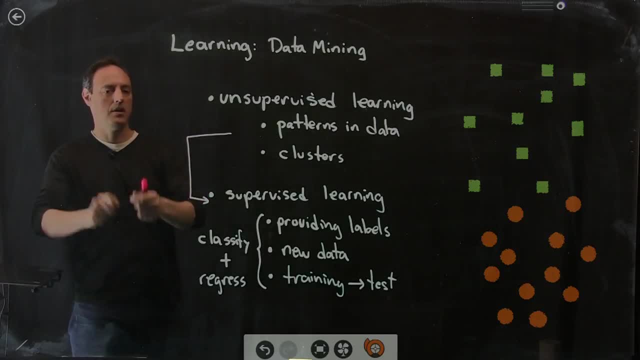 and, for instance, I could say: hey, these are green squares, these are orange dots, I've labeled them, so you know what they are. So you already know. there's two clusters, two types of data, And so the idea is, what happens if I have? 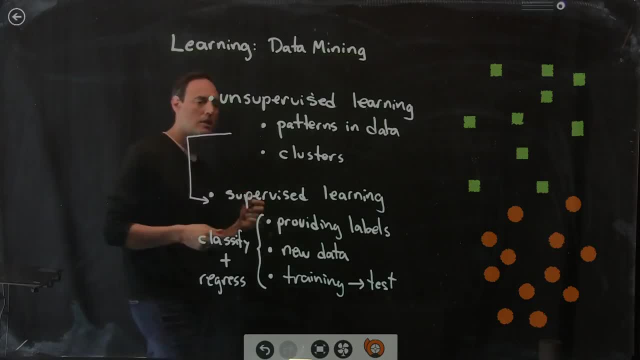 new data in the system. So, for instance, let's take a look at something like this: Suppose I have a new piece of data right there And the question comes. so this is something where I've already got my clustering. so now I wanna go down to my supervised learning algorithm. 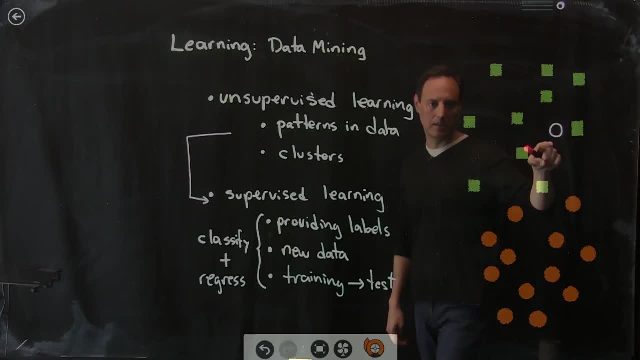 which is to say: what is this? If I give you a new piece of data and it sits right here, what is it? And, of course, from the naked eye, you'd say, well, I don't know. it's up here with all the greens. 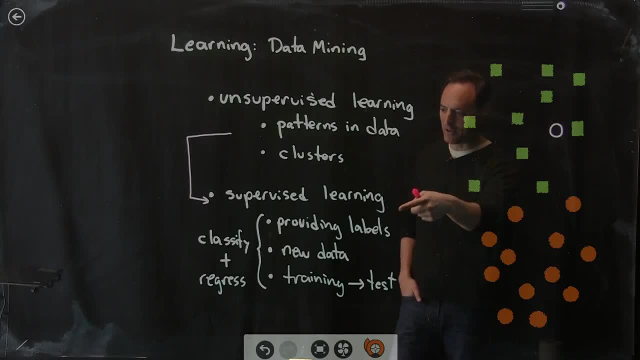 It's probably a green. So that's how that supervised learning would do. It would go right down to this classification, regression, And in fact, you might even say what classification and regression are really gonna try to do for you here in providing a training is to decide. 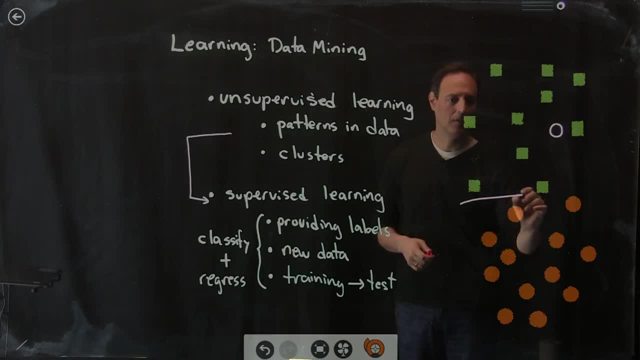 how to separate this data. So, for instance, you might separate the data like this: Anything above here is green, Anything below there are orange dots. So this example is very simple. So even if I do classification of that orange circle or this circle here, it's clearly above, here with the greens. 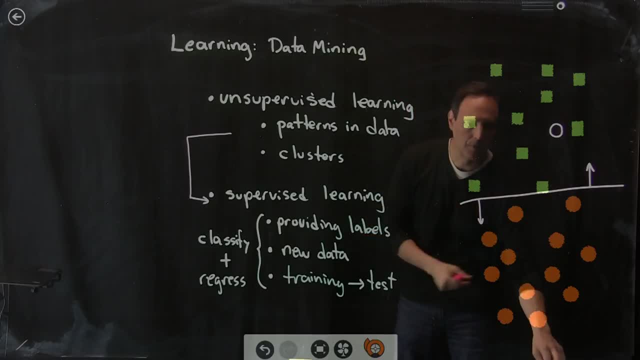 I would classify it as a green square. And if I had something down here, piece of data down here, let's say this X, and I say what is that X? Well, I'd say, oh look, it's actually sitting down there with the green. 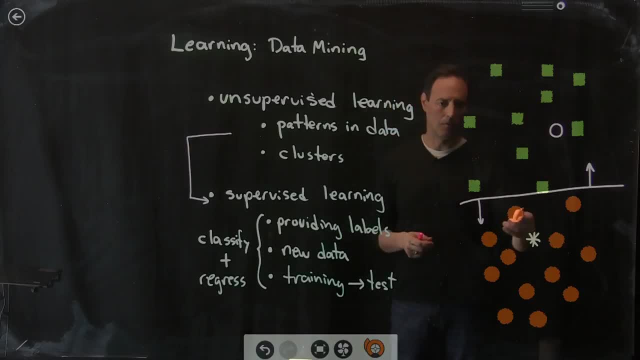 Well I'd say, oh look, it's actually sitting down there with the green. Well, I'd say, oh look, it's actually sitting down there with the green. I'm sitting down there with the cluster of orange balls, So I would label it as an orange ball. 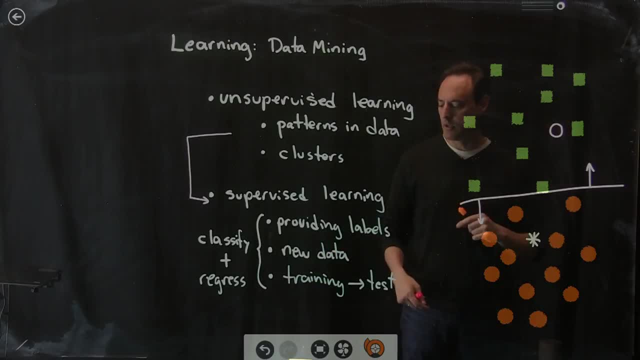 So that's the idea here is that you have a training set, let's say the green and orange, and now your test set are these new data points. So if I gave, for instance, if this was dogs and this was cats, if I gave you this new point, 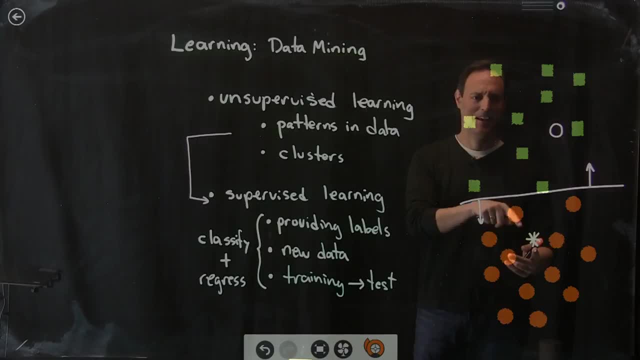 I'd say: oh, that's a cat. I think I said that was: let's say that's a cat. Let's make this up. let's say: these are cats down here. Let's say: and these are dogs up here, okay. 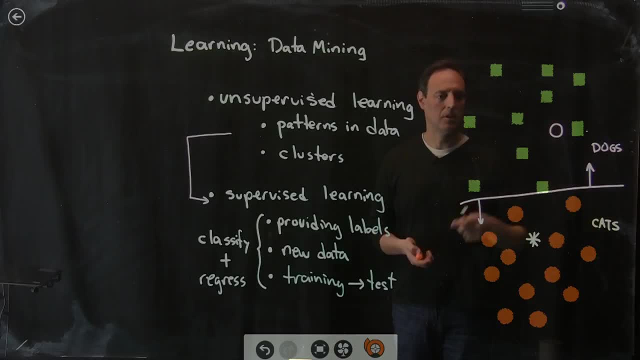 So then, any dots down here would be cats. any dots up here, sorry, cats down here, dogs up here, and that's the simple classification, okay, And again, you can get at these through these different type of methodologies. In this case, if you knew, it was dogs and cats. 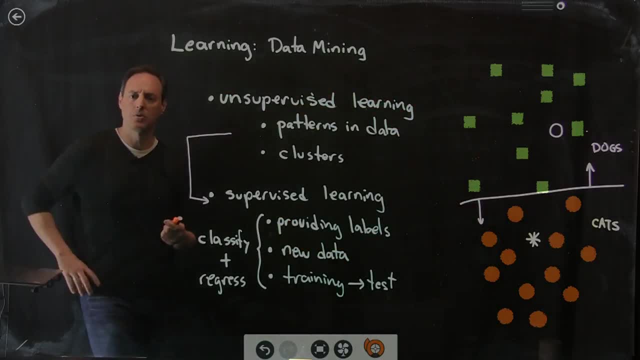 you would say, oh look, I can already know that there's two sort of types of data in there, so I'm gonna go ahead and classify it as such, okay, So this is kind of the general idea, and again, unsupervised. this is a really key concept. 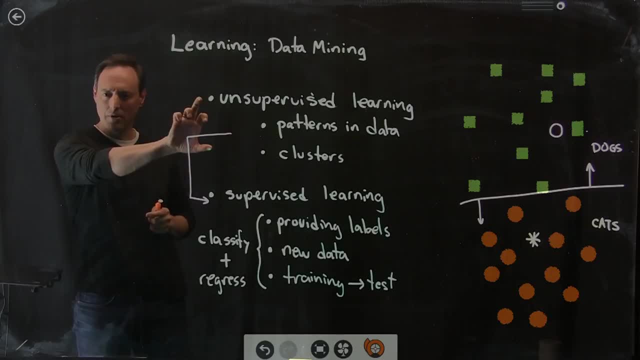 unsupervised, essentially for data that you don't know anything about. provides you a way of getting labels on your data, All right. so it's looking for clusters. You have to pick the number of clusters, but once you've done that, 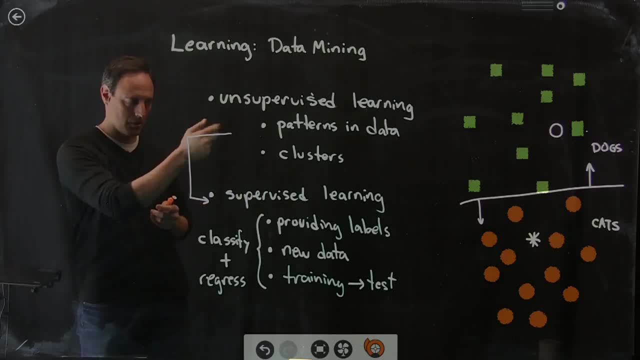 it provides you with labels on those so it belongs to cluster one versus cluster two. Then you could do things like use those as training sets to do classification and regression. okay, And in fact, ultimately, what this allows us to do is the very important thing. 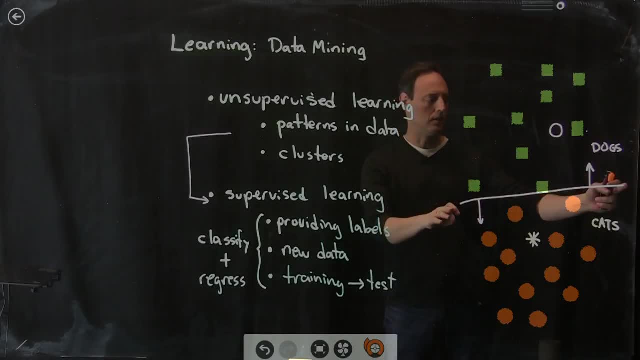 of drawing this line right here. This line here is essentially gonna be like my regression line, because it's giving me a mathematical formula for distinguishing between one type of data to another. okay, That's ultimately a lot of the goal of data and that's what we're gonna do with mining. 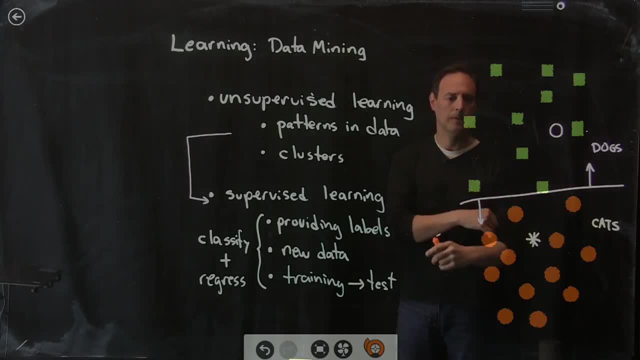 is to first look for clusters and then provide these lines of separation between the data. Now, this case is fairly easy, right? If we look at this case, everything separates nicely. Let's take a more sophisticated case and see what that would give us. 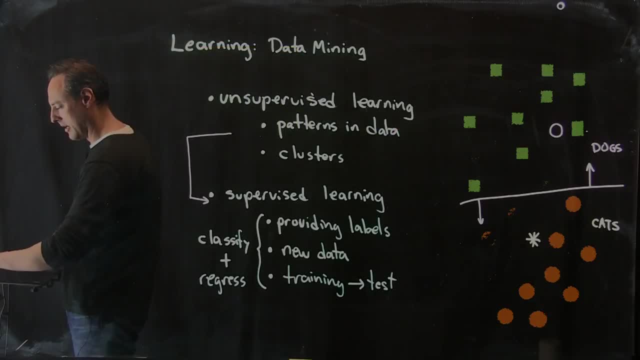 So I'm gonna erase this data. It's probably a faster way than I'm gonna do it, but fine, I'm gonna just erase all this, okay, And we're gonna come up with a new data set. This data set is not gonna be as clean as that one. 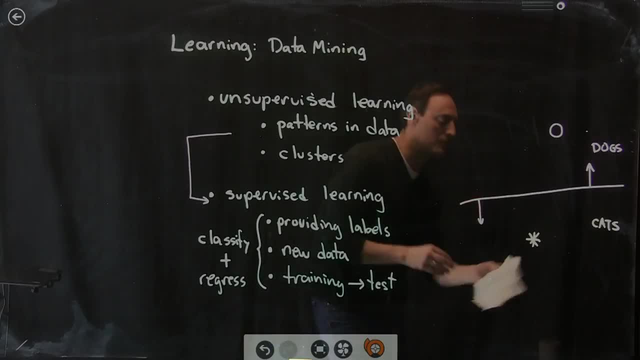 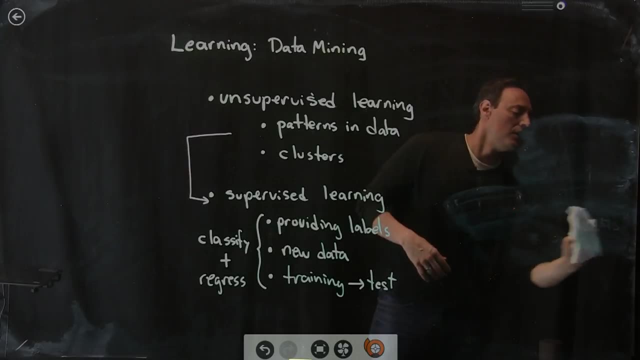 where I had everything separated. In fact- let me erase this line here- that we have our classification line. So in this case that I drew- and of course, oftentimes in textbooks, you always see these nice cases where everything separates out nicely. 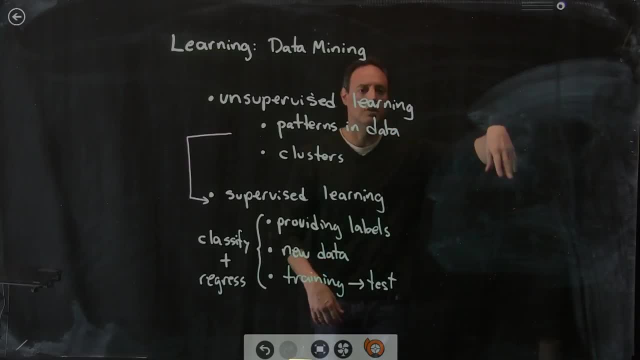 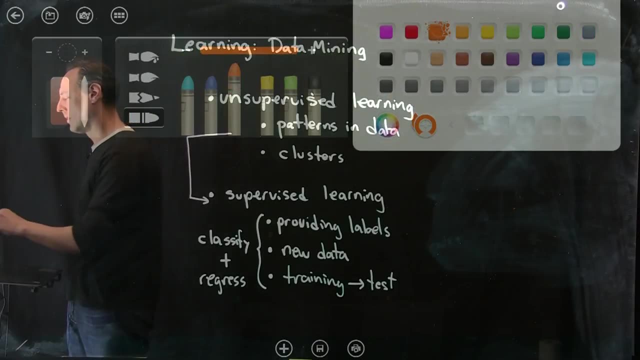 and there's no problem, and it's almost through the naked eye. You can make these distinctions about what they are, But in a lot of cases it's a little bit more complicated than that. So let's go ahead and draw some of these orange circles. 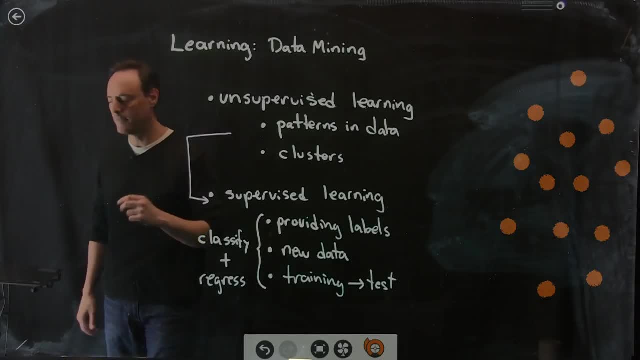 And let's just say that's my data, all right. And then I can say: well, what if I had another type of data? Then I could ask: do you think you have a shot at having a nice regression line that would separate the orange from the green right? 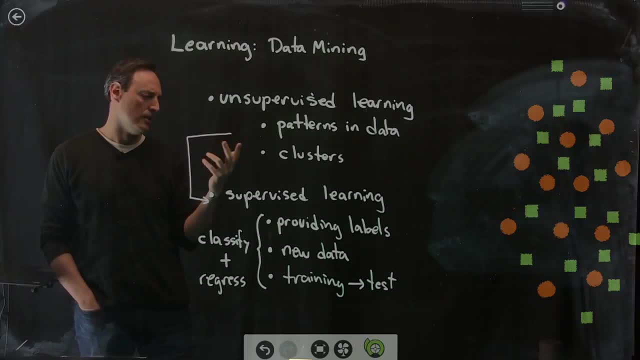 And that's a lot of times when you get data where the data analysis tricks don't work so well. But sometimes it's all about how do I get this down into that representation in the first place, And this is where something like principal components plays. a big role is in this sort of projection space. 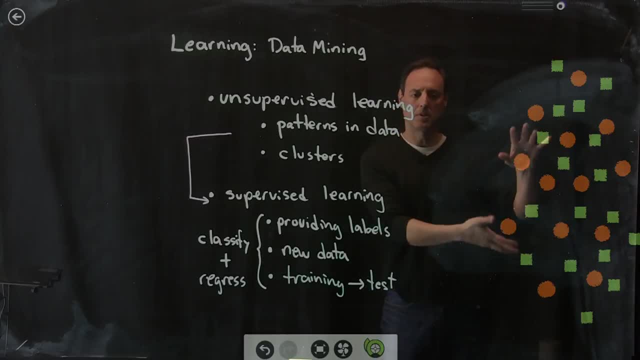 of where I've put my data. is there maybe a more clever way to represent the data where it does separate out, versus something like this where clearly there's no way? if I gave you a new set of data, let's say right here and I ask you, what is that? 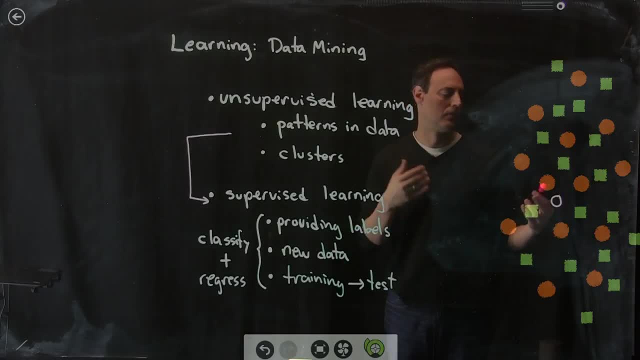 You would not be able to say with any kind of accuracy that this was an orange ball or a green square, because in fact it sits there in a sea of orange and green. So these are the kind of ambiguous types of things where your clustering isn't gonna give you. 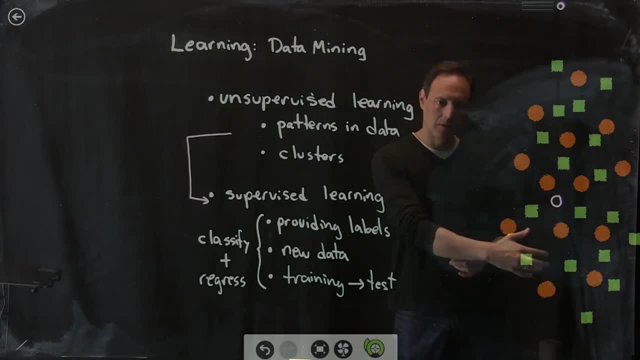 a good separation. Even if you label these data, it's clear it's not gonna give you a good separation. So in the data analysis here there are serious, let's say, drawbacks that you might encounter with such type of data. okay, 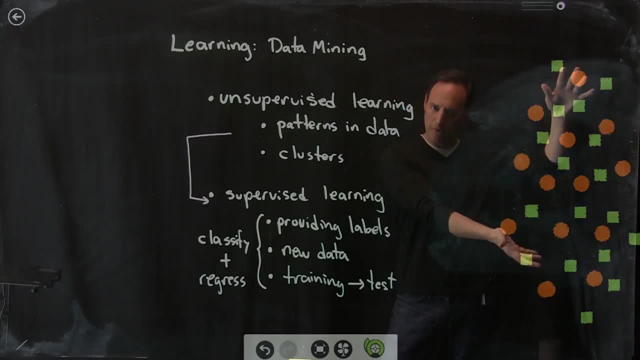 So that's, but this can represent realistic data that you would have in practice, and so it's important to understand that a lot of times you're gonna see things like this, okay, So we've given you one case where it's a nice separation. 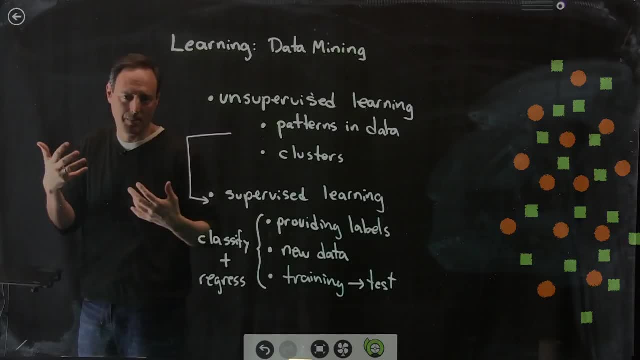 one case where it's not a nice separation, Let's do what's more typical, which is kind of some hybrid in between, where you get some separation but you get some mixing, And so let's go ahead, and I'm gonna show you one example of that, and I always think of this. 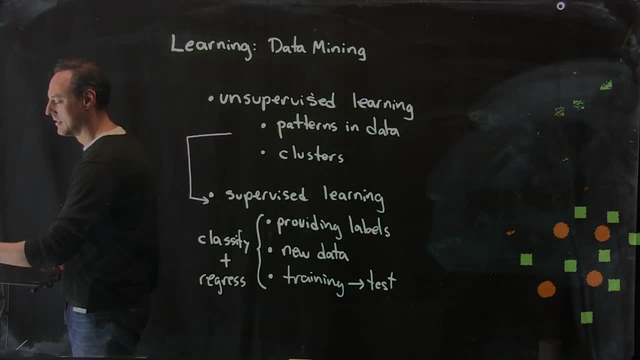 as sort of being. this is kind of what you more get in practice than anything else. All right, got all that erased, Let's go put some more dots down. Okay, we're gonna go back to green squares, So I might have some things out here. 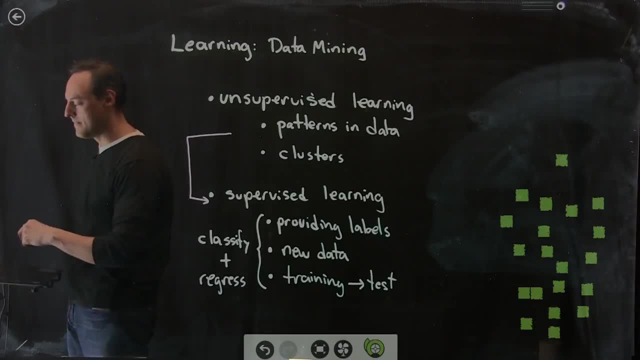 Nice cluster of green squares, All right. and then I might have my orange data as well. There's the orange and, Okay, let's look at this example here for a moment. So now, in this case, you clearly see that most of the greens are below most of the red oranges. 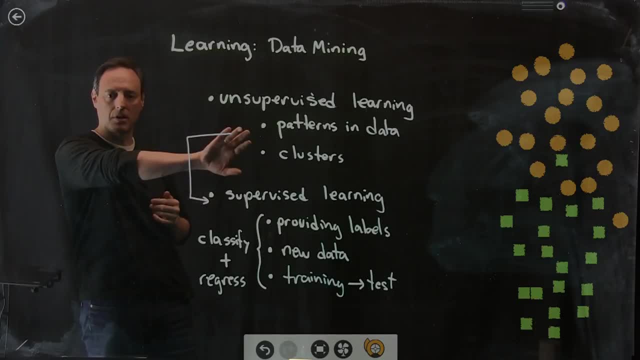 are above. This is a nice separation. so if you were to do some kind of clustering analysis and you didn't know the number of clusters, but if you did manage to pick two clusters, what you would find is probably something bunched up there in the orange. 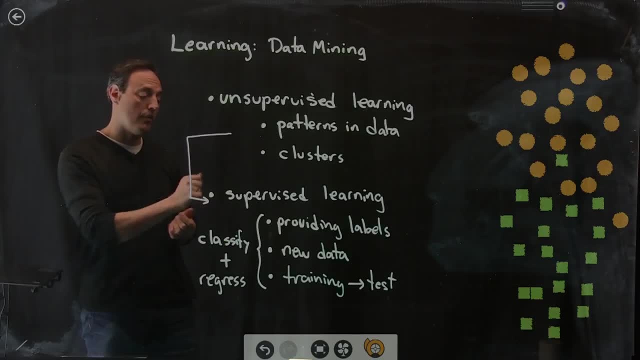 something bunched down on the bottom in the green, or even if you were to do a supervise, which is, if you labeled these things, you would see this thing and say: here's a bunch of orange balls, green squares, and what I wanna do is these two things here. 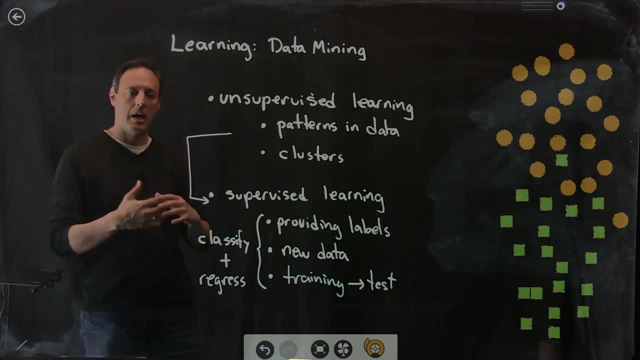 at the end of the day, classify regress, In other words, figure out how do I wanna classify new data and how do I draw a regression line which ultimately leads me to a way to separate the data, In this case, here you might think that the best. 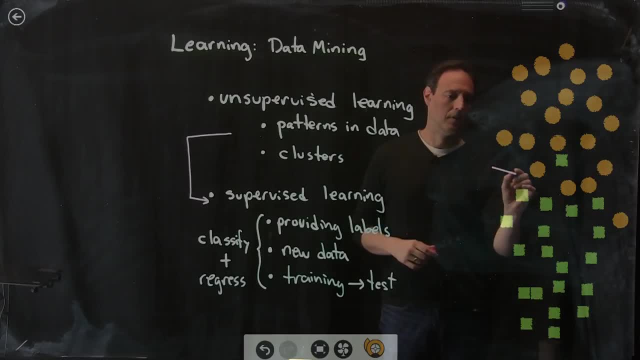 separation line. I don't know, let's just draw something. might be something like this. So again, anything above here is an orange ball, anything below here is a green square. So in this scenario you get a nice separation. but notice: 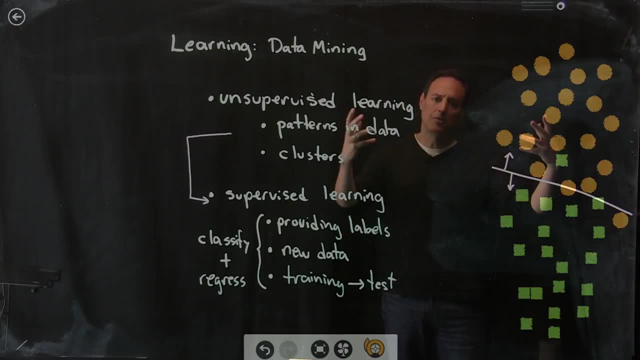 you're gonna make mistakes And, by the way, that's the general thing. What you hope to do in data analysis- even looking for data mining and patterns in your data- is that. what you hope to do is get the right trends, maybe even get accuracies in the 80s- 90s percents, right? 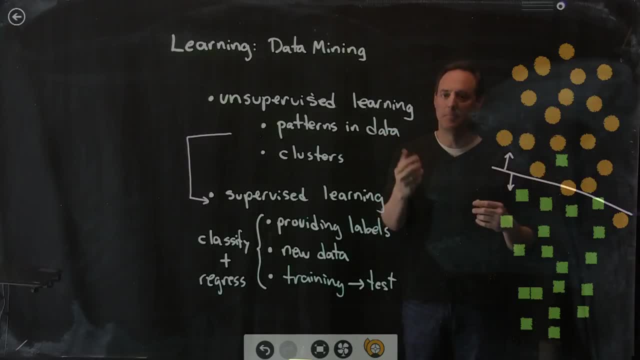 That would be fantastic. Even if you can sometimes get above coin flip, it's pretty good. So if you can do better than just guessing 50%, maybe you find that your accuracy is only 55%, but that's still better than just a pure guess. 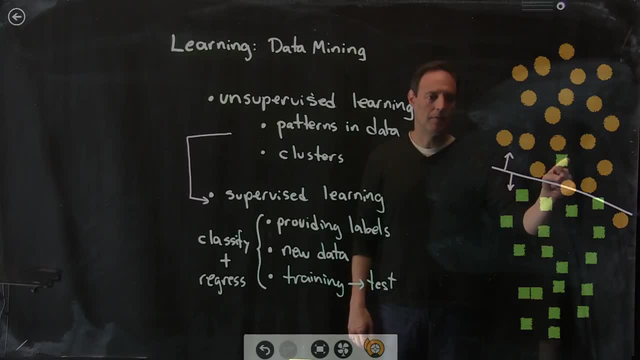 But something like this: clearly you're gonna make mistakes. Okay, you already see. Right here I have this green square and that green square gets misclassified In this algorithm. it would say that this green square is actually an orange circle, and that's wrong. 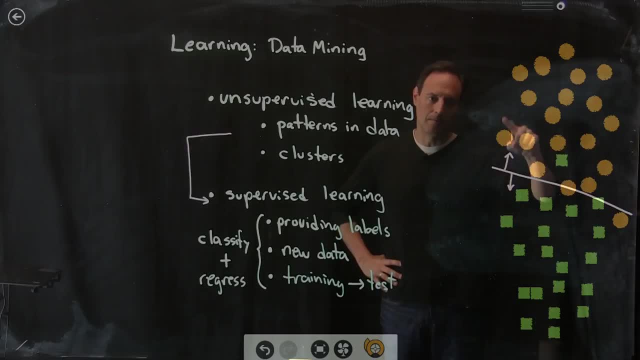 So you've made a mistake. However, you got most of the other ones right Now. on this side over here, you get a lot of the green, but look at this guy right here that gets misclassified as well. So this one here gets misclassified. 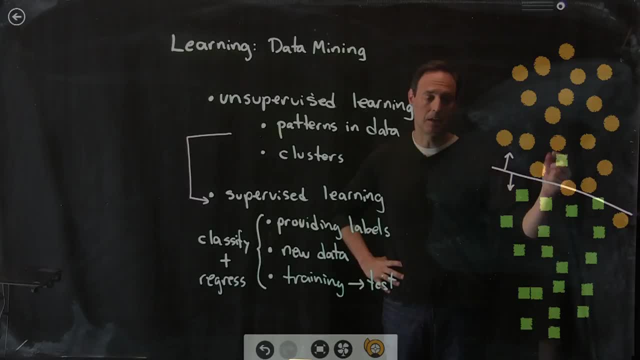 as a green square. so you've made a mistake on this side. you've made a mistake on this side, and also things like this, this one here which sits right on that boundary line. it doesn't know quite what to do. 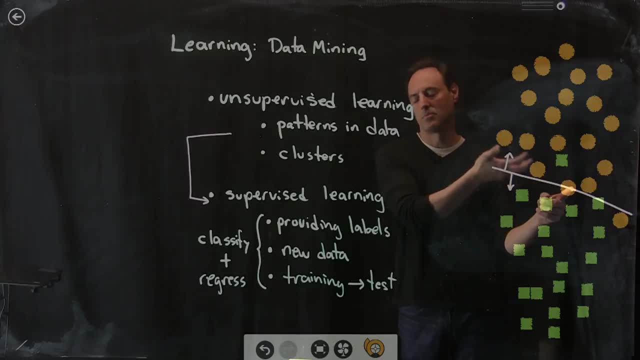 Basically, the algorithms has double precision accuracy. so at some level of 10 to minus 16, it's gonna be on one side of the line or the other and it's just gonna simply get classified as being one of these or one of these, okay, 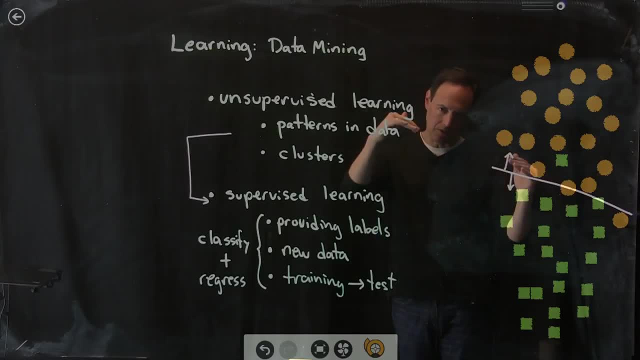 But these points are very interesting because they're right at the border of your decision space. On one side you're gonna get one way. on the other side, you're gonna get another way. So that's a kind of a more generic thing. 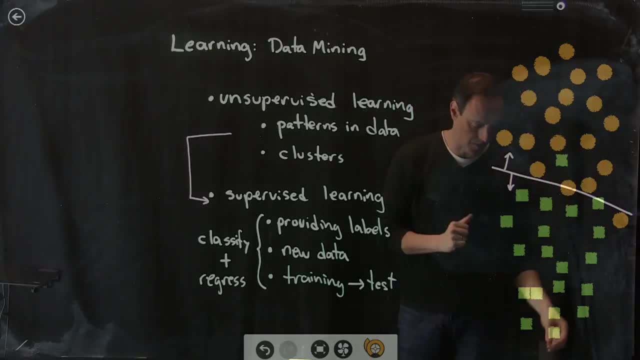 You're gonna make mistakes. You're not gonna get perfect classification. Now, the one thing I'm gonna highlight here is that I think one of the biggest dangers in data analysis is this danger of overfitting your data. This can happen a lot in the supervised learning algorithms. 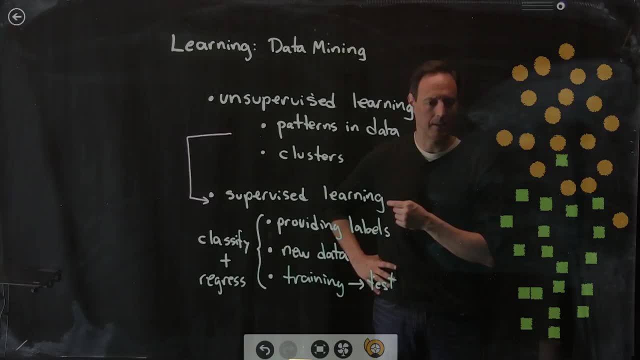 You have to be really careful. I'm gonna talk about this concept of cross-validation. I'm gonna illustrate it here. If I wanted to do some kind of classification on this data- and this is my training data- and I want to do a perfect classification task- 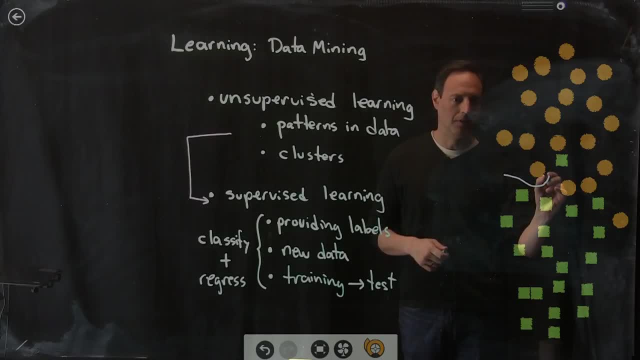 I might draw something like this: Let me see if I can do it here, Go around here And I could say: hey, look at that, If that is my decision line, my classification, I'm gonna get everything perfectly right. The problem with something like this is: 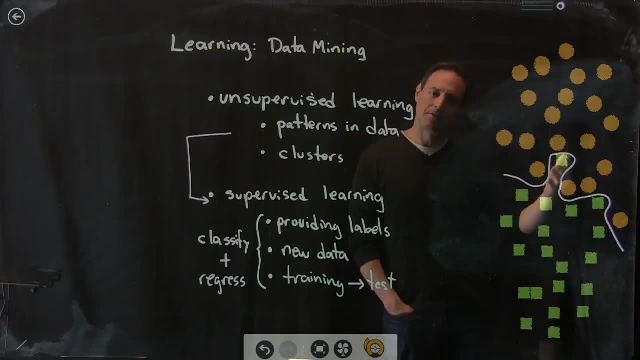 I can take any training data and if I want to generate some sufficiently complicated curve, I'll get 100% accuracy. So it's gonna start talking about the idea of cross-validation, which is: how well does this hold up when I put new data to it? 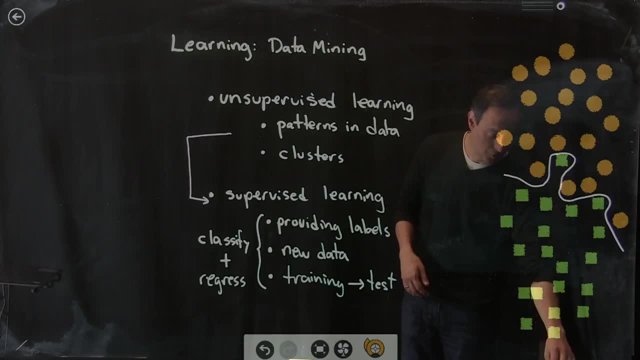 Okay, so the idea of cross-validation is: it's the idea of cross-validation which is: how well does this hold up when I put new data to it? Okay, so the idea of cross-validation is: it's the idea of cross-validation which is: how well does this hold up when I put new data to it? 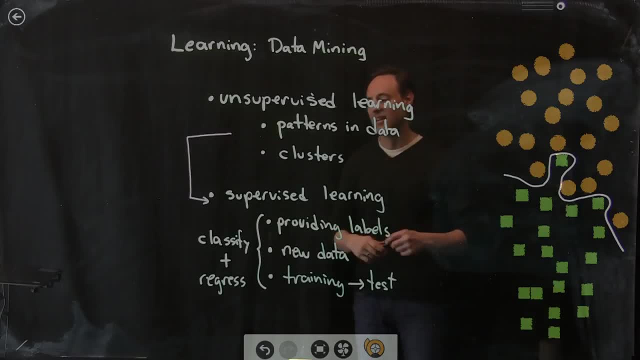 Extremely important. perhaps maybe the most important thing to take out of all of this is: you better cross-validate. How would a cross-validation procedure work? And, by the way, always, All right, always you cross-validate. Never miss doing this step, okay. 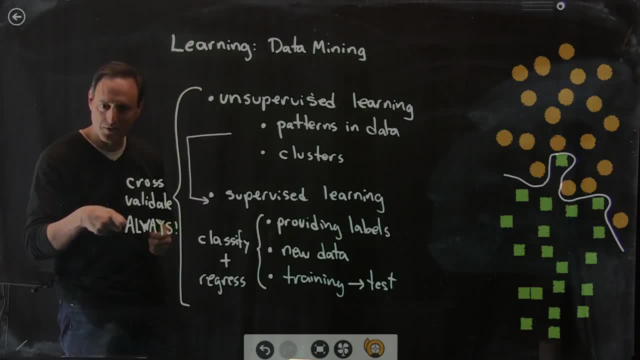 Never miss doing this step. okay, Never, ever miss doing this step. If there's anything you wanna write down here, always cross-validate. So how do we think about it? Well, cross-validation says the following: How about I do this? 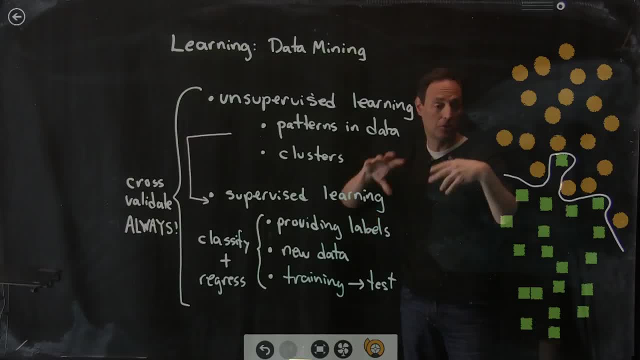 Since I'm gonna provide labels to data and this is gonna be my training set, what I'm gonna do is take all my data that I have. suppose I have 100 orange balls and 100 green squares. Suppose I had that. Well, one thing I could certainly do is take 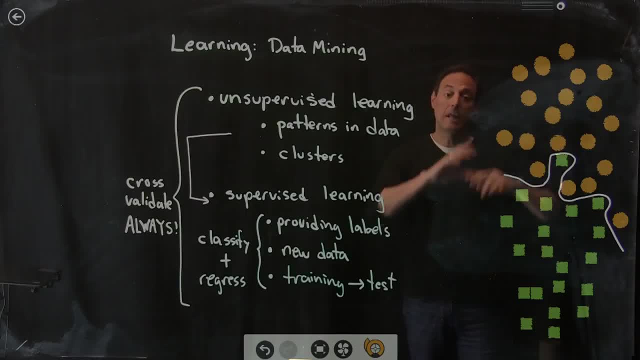 80 out of the 100, randomly chosen. I'm gonna take 80 randomly chosen here, 80 of the 100 randomly chosen here. So I'm gonna take 80% and I'm gonna be have that be my training set. 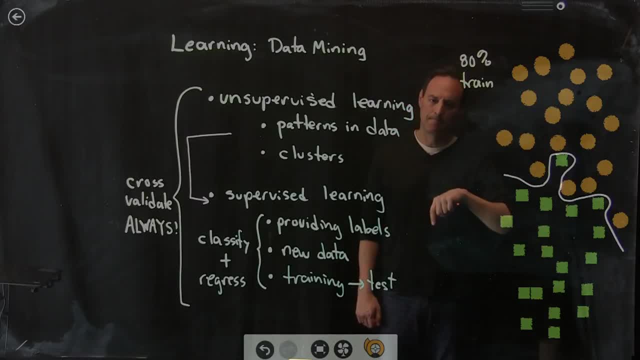 So I'm not gonna train with all the data I have. I'm gonna train with 80% of it. But what I'm gonna do now to go test new data is I'm gonna hold the 20% I withheld is gonna be my test data. 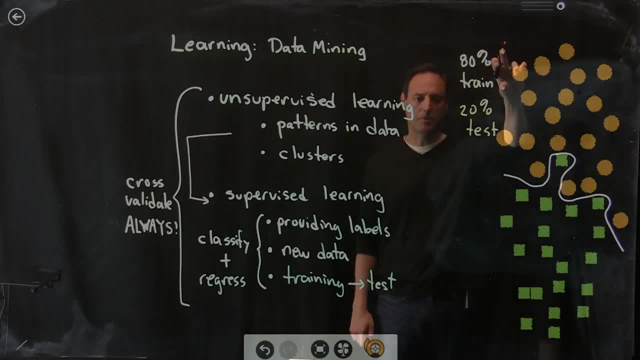 Okay, So I take 80%, I test with 20% And I'm gonna draw a decision line for every time I do this. So I'm gonna test it and I'm gonna get an accuracy. So I'm gonna get some kind of accuracy score. 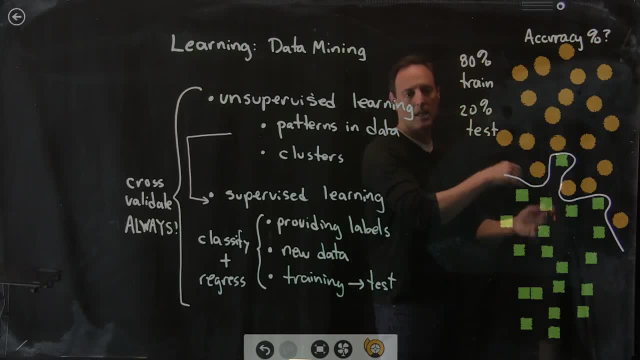 But then once I get an accuracy score, let's suppose I do this and I get some decision line and I get an accuracy of 95%. What I'm gonna do is: maybe I just got lucky, Maybe when I picked I didn't pick this problematic guy. 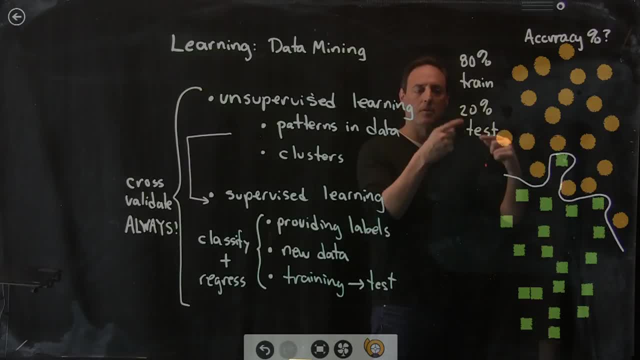 here and this problematic guy over here. So I'm gonna shuffle. I'm gonna take a new 80% and test on that remaining 20% And I'm gonna do this randomly again. Take a new random 80% test on the other 20%. 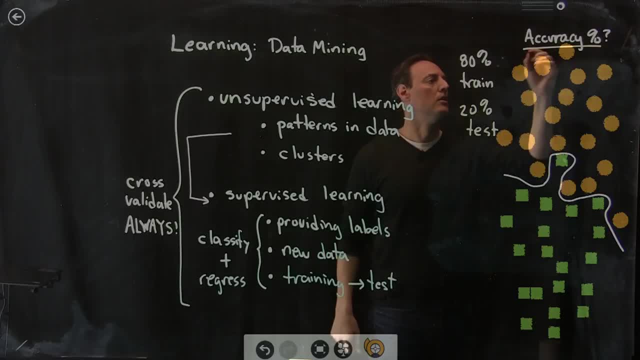 A new random 80% test on the other 20%, And what I'm gonna do is keep track of my accuracy as a function of these random trials. And what ends up happening is you no longer get curves like this. This curve was very specific to this exact data pool.